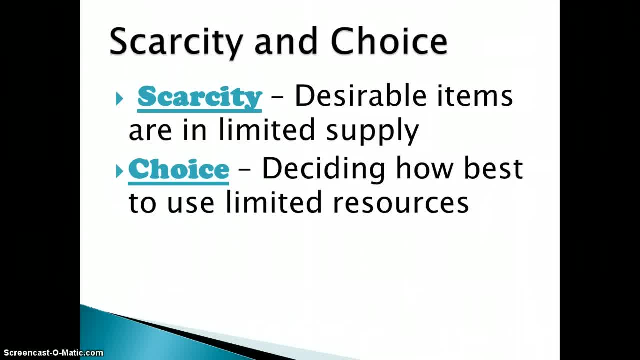 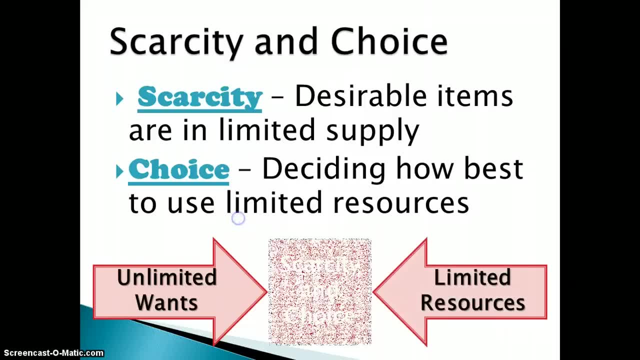 That what we want is limited, but our wants themselves are unlimited. So in a world where we have unlimited wants but limited resources, we have to make a choice, because everything that we want doesn't exist, And so we have to figure out a way to allocate resources so that we get the most benefit at the least cost. 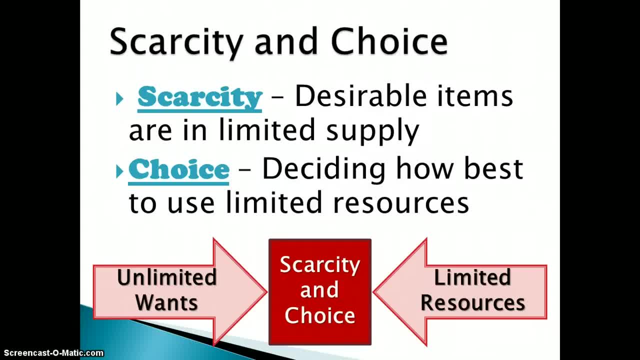 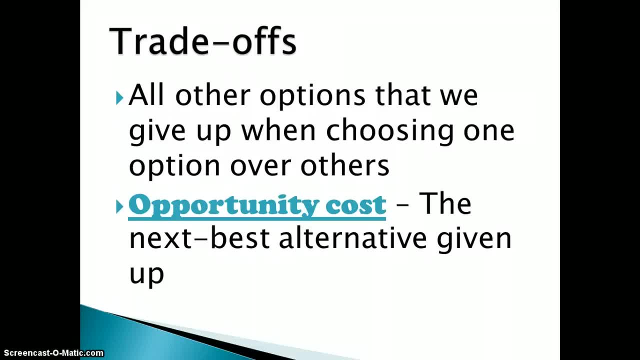 And so we have to make difficult decisions, And because we have to make difficult decisions, we have to be able to identify what the right decisions ought to be. Our whole life is built around trade offs, And so when we have to give up something, that's what we call an opportunity cost. 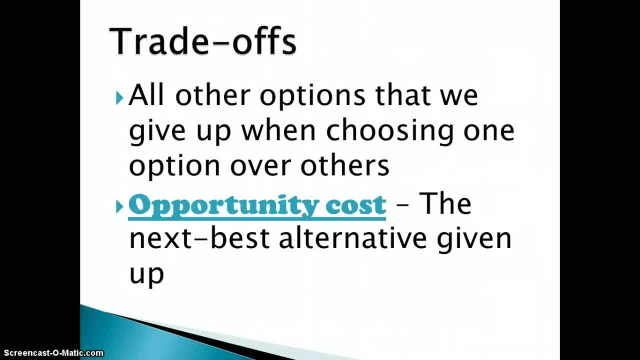 So anytime that I choose to do one thing Or purchase one good at the expense of another, Then the next best alternative is what I would identify as being my opportunity cost. So if I choose to study for a test instead of watching television, and that would be my next best thing, 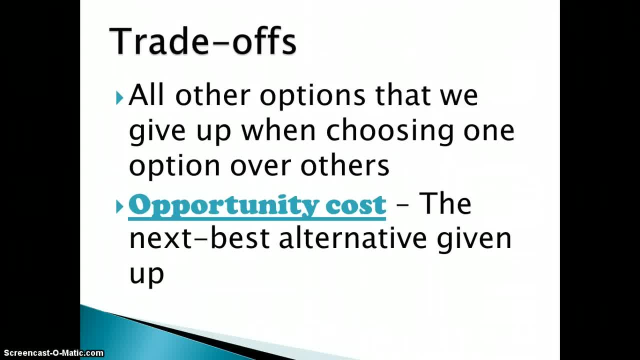 Then the opportunity cost of getting a good grade would be the time that I could have spent watching TV. Another example might be if you're at a restaurant and you're trying to decide what to get Off of the menu and you would like two different meals, but you can only order one. 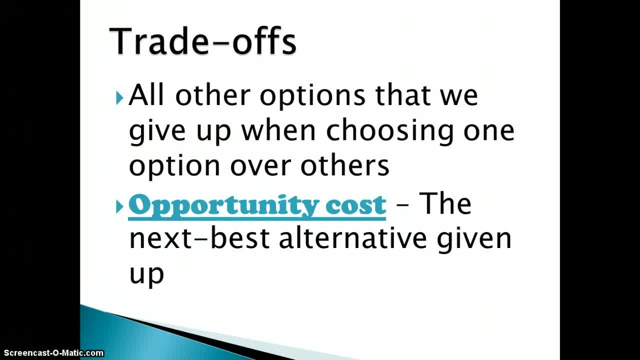 Then the opportunity cost of the meal that you eat is the meal you gave up. So we live in this world where we're constantly making choices and we're giving up one thing for another. So when we look at something like a production, possibilities curve. 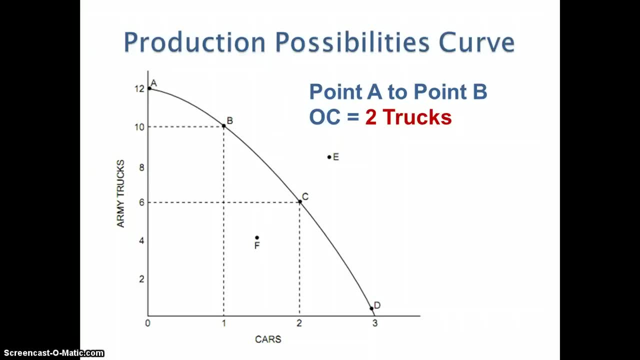 We can begin to identify what opportunity cost is and put a number on it. So in this example we've got two products we could be making. We could be making army trucks, We could be making no cars, And the production possibilities curve tells us all of the possible combinations of trucks and cars that can be produced in this economy. 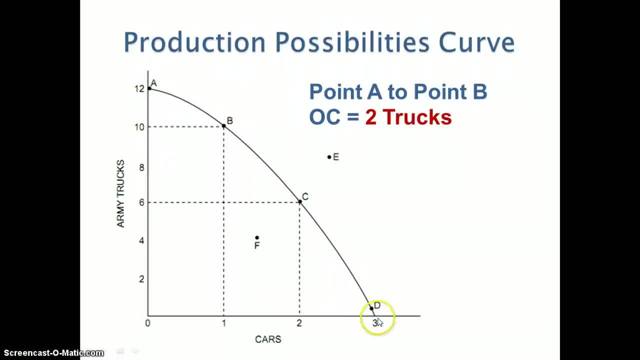 So we could make twelve trucks and no cars. We could make three cars and no trucks Or any other combination between those. So point B would say: ten trucks and one car. Point C would be: we could make six trucks and two cars. Now point E is not attainable. 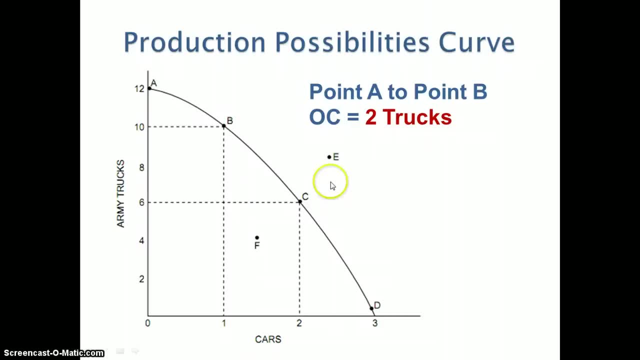 We don't have the resources and the ability to reach that yet, unless there's some sort of economic growth. Whereas point F is something we could make but it's not considered efficient Because we could be making more of both cars and trucks If we were producing at point A, where there are twelve trucks and no cars. 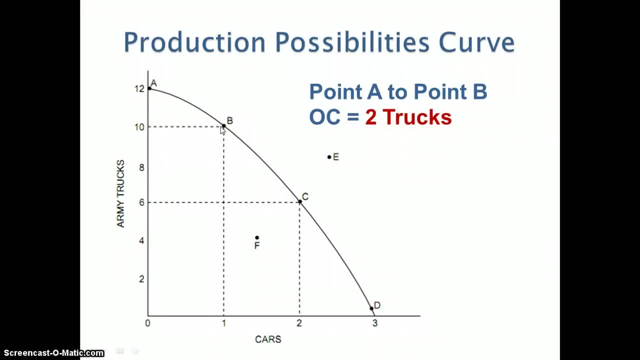 Then moving to point B would leave us with an opportunity cost of two trucks, And the way we can figure that out is by saying: if I give up or if I produce one car, I'm giving up two trucks. So the opportunity cost of producing one car is two trucks when we move from A to B. 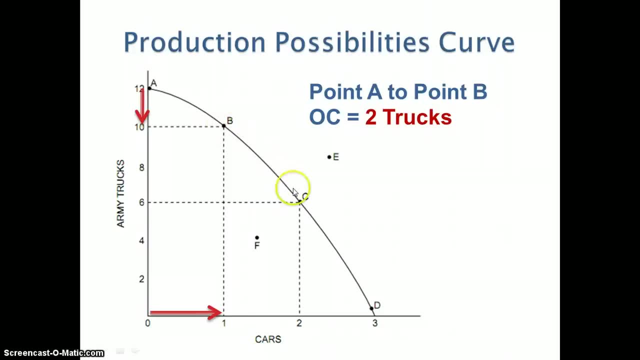 If I was to move from point B to C, Then the opportunity cost for one car is equal to four trucks. In order to get one car, I gave up four trucks, And if I was to move from point C to point D, Then I would give up. 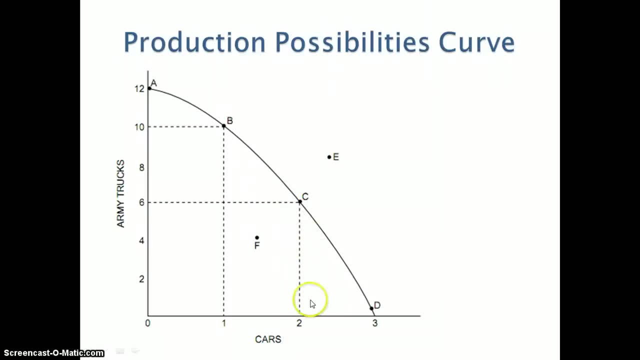 I would be giving up roughly six trucks for one car. So the opportunity cost, moving from C to D, of adding one car is six trucks. Like I said, point B is efficient. It is maximizing our production. Point F is inefficient Because I could be making more of both. 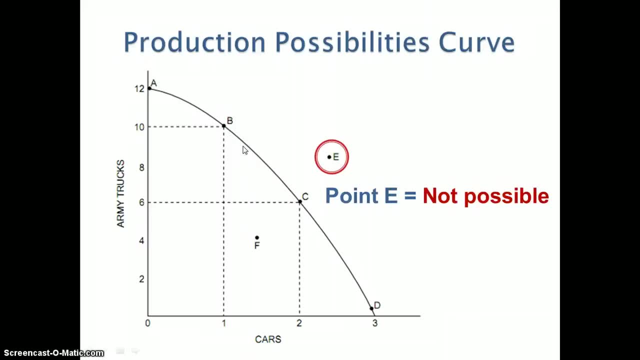 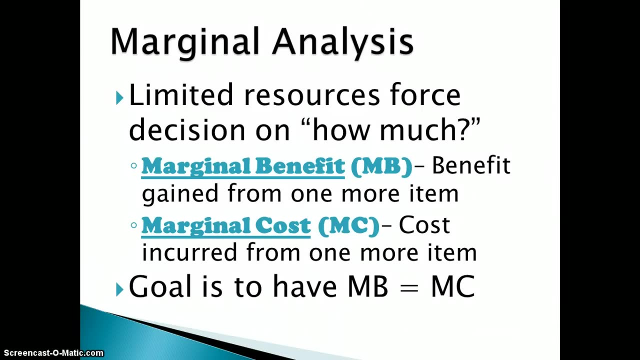 And point E is not attainable unless there's some sort of long term growth that occurs. This other concept is one of more common. This other concept is one of marginal analysis And in microeconomics in particular, we constantly talk about things as on the margins. 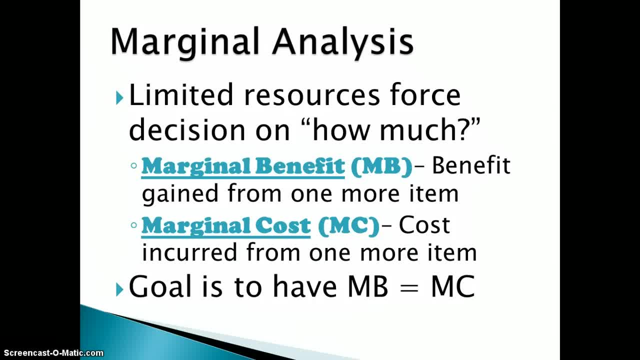 We want to know whether or not decisions we make make economic sense, And so we look at marginal benefit and marginal cost. Anytime you see marginal, what it's talking about is the additional change that occurs by the change of one factor or variable. So, with marginal benefit, 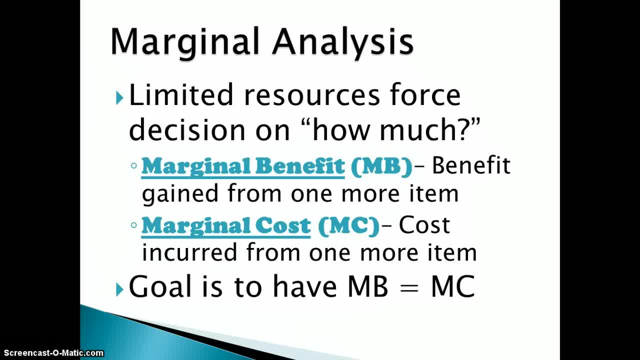 It's the additional happiness I get for one more item, And marginal cost is the additional cost I receive for doing one more thing. So an example would be like eating donuts: If I eat a donut and I get ten units of happiness for the first donut. 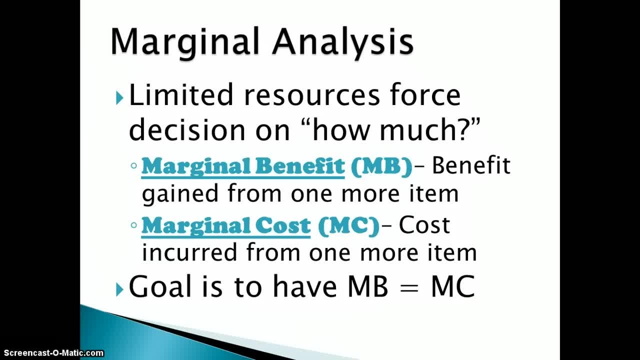 And it only costs me one unit of unhealthiness, Then that would make sense for me to eat, Because I get more happiness than the cost. The second donut I eat will make me happy, But by not as much, Because I've already had the first donut. 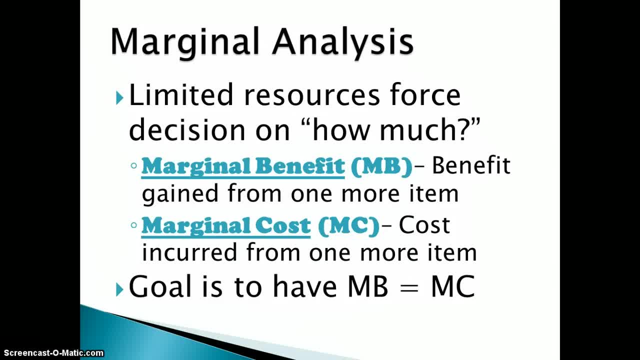 So maybe it only brings me eight units of happiness, But that second donut also kind of adds to my health cost. So maybe the second donut leads to two Negative two for my health And we could keep eating donuts And the donuts would make us happy. 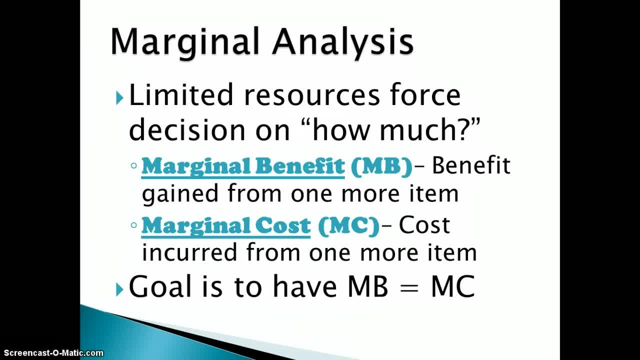 But the additional happiness would begin to dwindle, The marginal benefit of each additional donut would begin to get smaller, And the cost of each additional donut would begin to get larger, And so we would stop eating donuts when the marginal benefit 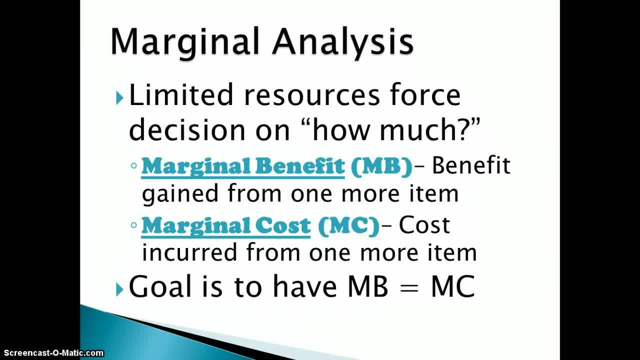 The additional happiness of the last donut I eat Is equal to the marginal cost of that last donut. So as long as marginal benefit is greater than marginal cost, It makes economic sense to take an action Or purchase a good Or consume a good. 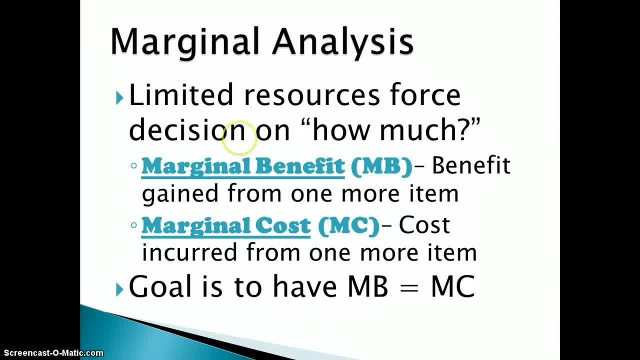 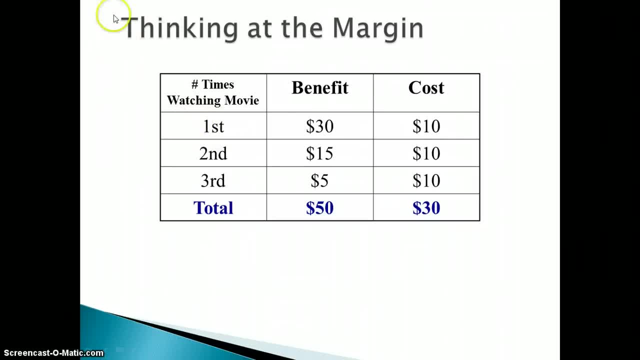 When marginal cost is greater than marginal benefit. You should stop. So if we think at the margins And we look at watching a movie, We can say: the first time I go to the movies I get $30 worth of happiness And it only costs me $10 to get in the door. 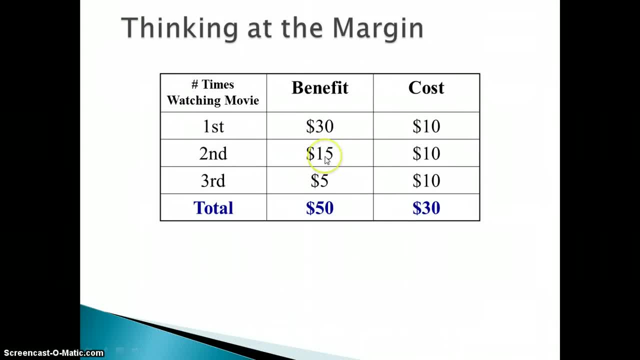 If I watch the movie a second time, I might get $15 worth of happiness. There's some stuff that I saw That I really liked I wanted to see again, Or maybe there was something I missed That I caught the second time. 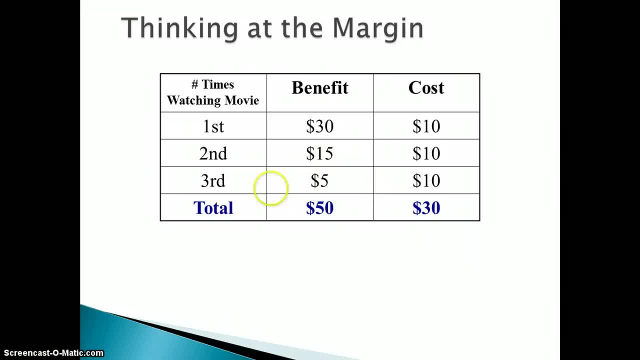 But it's not like watching it for the first time Because I know how it's going to end. So I get a little less benefit, But it still only costs me $10.. The third time I get $5 worth of benefit. 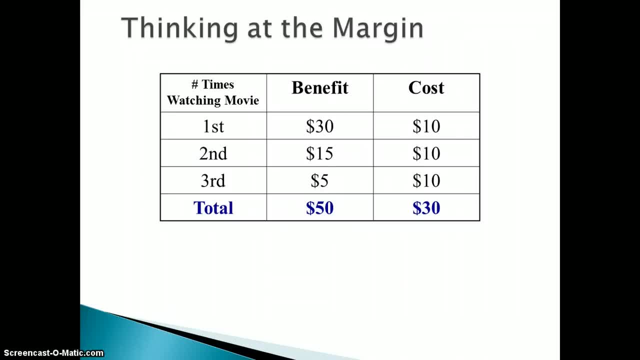 Because I know all the jokes. I know exactly what's going to happen. There's not a whole lot new to me, But it's still kind of enjoyable. But it costs me $10 to get in the door. In that case We look and we say 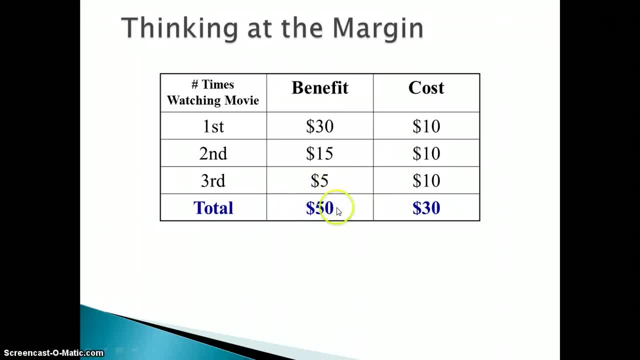 Well, total benefit, I got $50 worth of happiness Out of watching the movie three times. It only cost me $30.. So when you're looking at total benefit, It seems like Okay, Going with the third time to the movies. 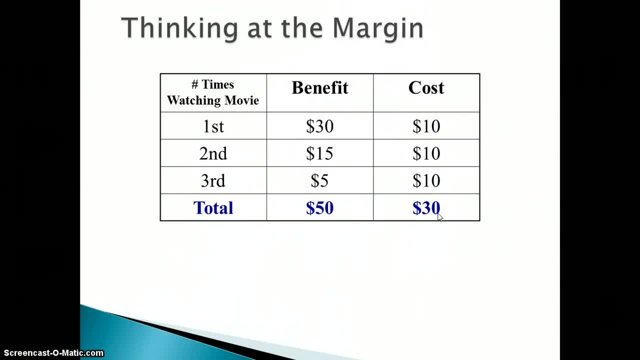 Makes tons of sense, But the reality is That that third time Was not cost effective, Because it cost me $5 to see it. Or I got $5 worth of happiness But it cost me $10 to see it, So that's. 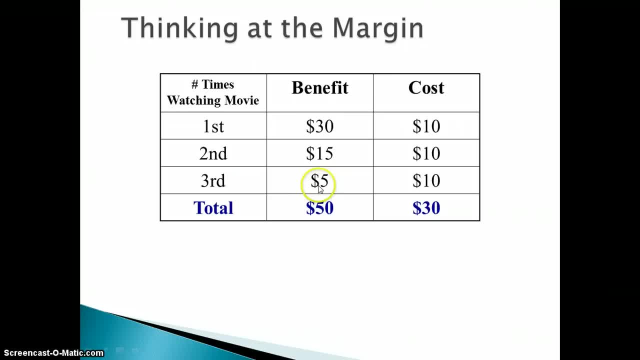 That's really, I'm losing $5.. So in that case, I get $5 worth of happiness, But it costs me $10 to see it. So that's, That's really. I'm losing $5.. So in that case, 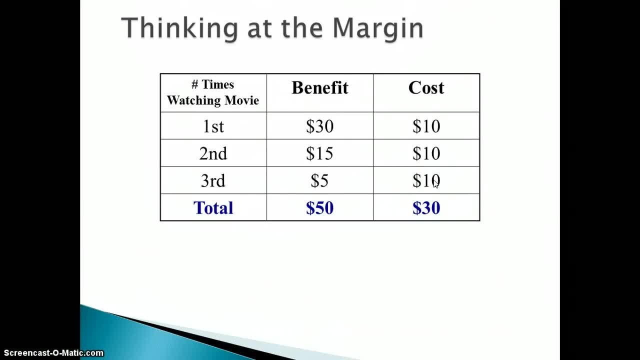 Looking at marginal analysis, Despite the fact That my total benefit Out of all three times I go see the movie Is greater than my total cost, That third time I watch the movie Is not economically viable, And so I will only go see the movie. 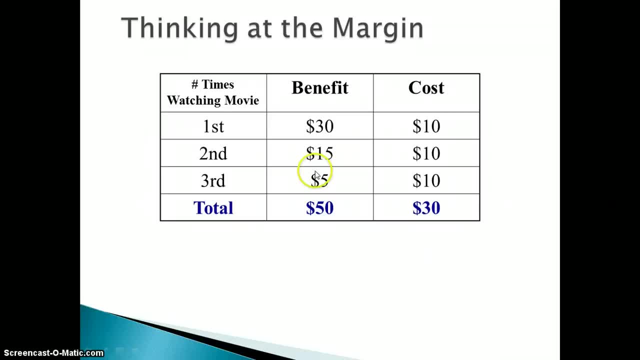 Twice. The last concept We want to look at Is comparative Versus absolute advantage. When we say That somebody has An absolute advantage, It means That they can Get $50 worth of happiness. So that's, That's really. 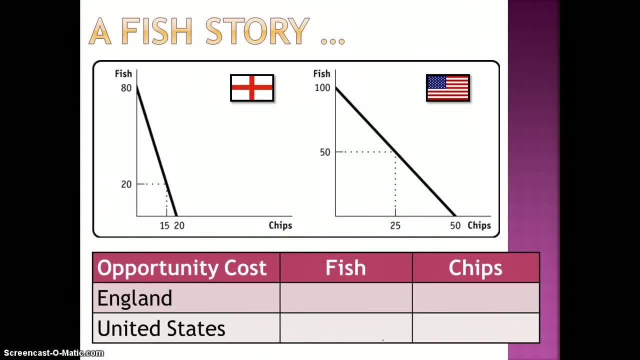 I'm losing $5.. So in that case, Looking at marginal analysis, Despite the fact That my total benefit Is comparative advantage, It means That they can Make more Of something Than somebody else. And When we talk about, 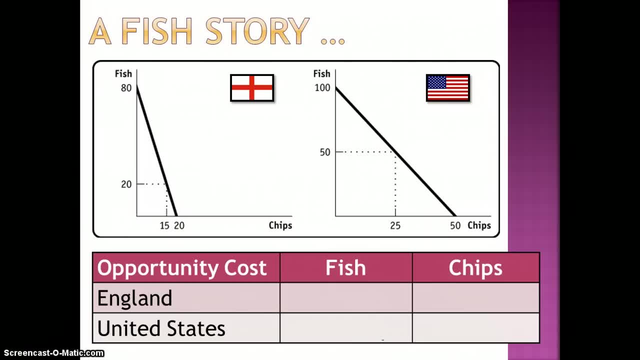 Comparative advantage. What we say Is that It is The opportunity cost Is lower For one person To produce a good Than another person. So let's just Take a quick look At an example. We'll say: 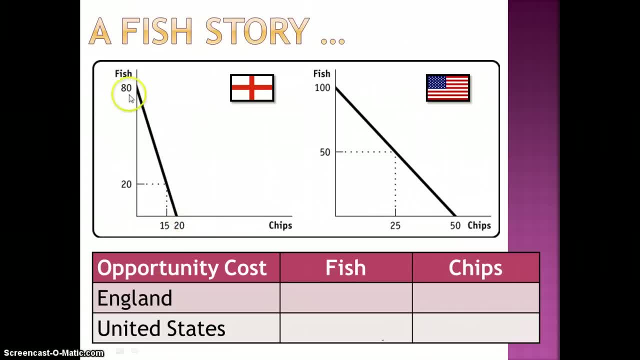 A fish story: Fish and chips. If we look At the data That we've got, We find That if You're in England, The English- We can produce 100 fish And no chips, Or 50 chips. 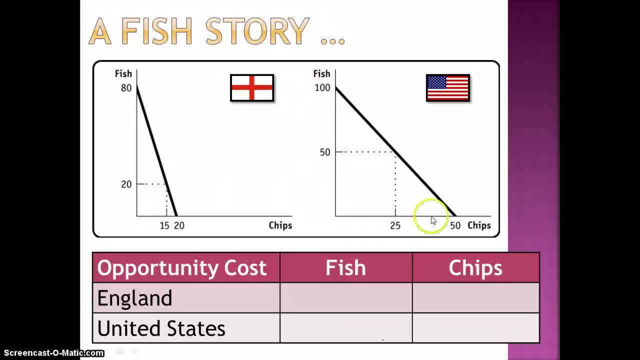 And no fish. So these are Our two production Possibilities, Curves And every combination In between. If we're trying To figure out The opportunity cost For England, Then we could say The opportunity cost Of making. 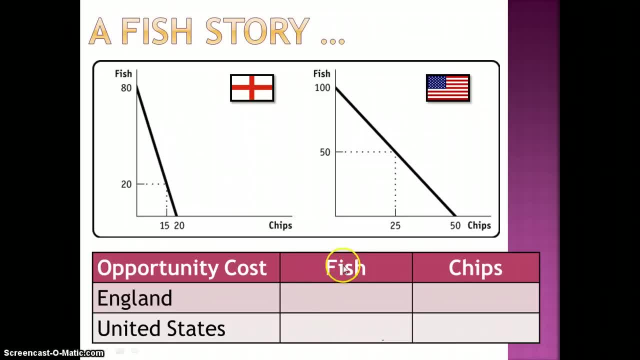 Fish Is How many Chips Per fish Do I give up? In this case, If I make 100.. Fish And no fish, I could Make 20.. Chips: I could have had 80.. 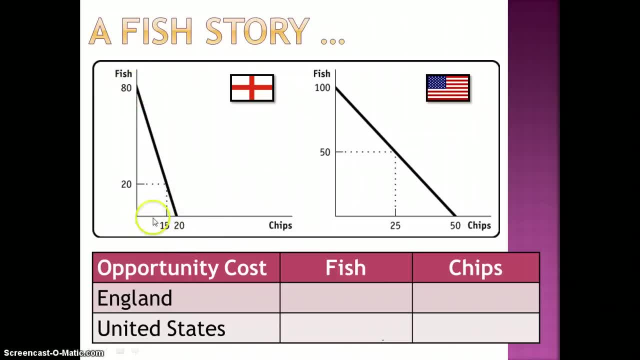 Fish. So if I choose To make 20. Chips And no fish, Then I That's One decision. The alternative Would be 80. Fish And no chips, So I would say That 20.. 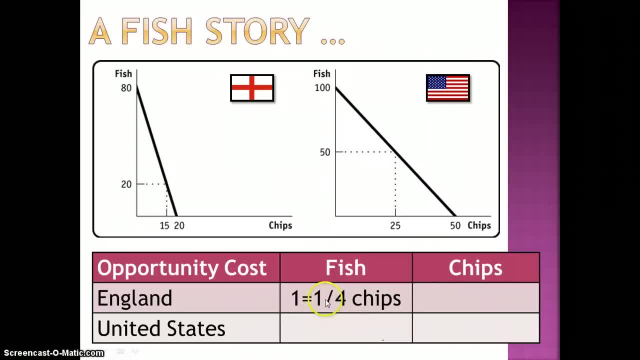 Fish Per 80. Chips- Sorry, 20. Chips Per 80. Fish. I'm giving up One quarter Unit Of chips. Their Opportunity Cost Of making Chips Then is How many? 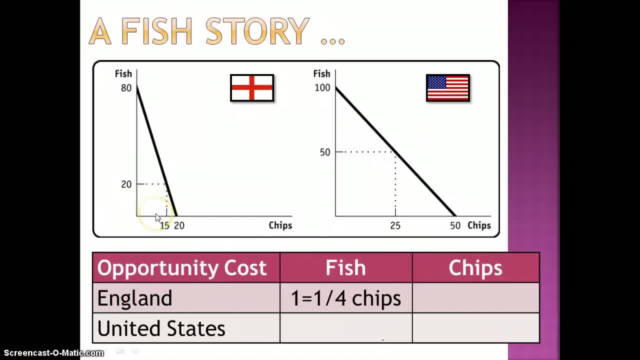 Fish. Are they Giving up Per unit Of chips Created? The good news Is that Once you Calculate One opportunity Cost, The other Is the Inverse. So if The opportunity Cost Of making 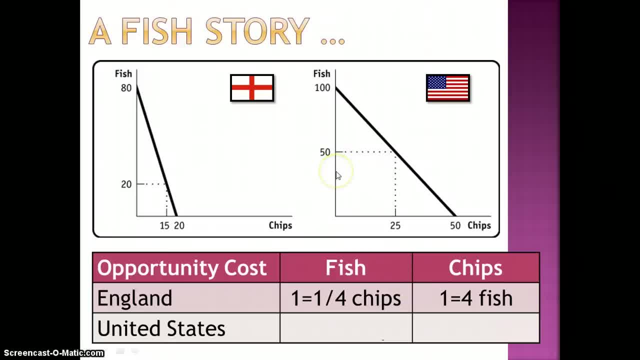 Fish For the US, Then The Opportunity Cost Of making Fish Is that They They give up 50. Chips If they're To produce 100. Fish. So the Opportunity 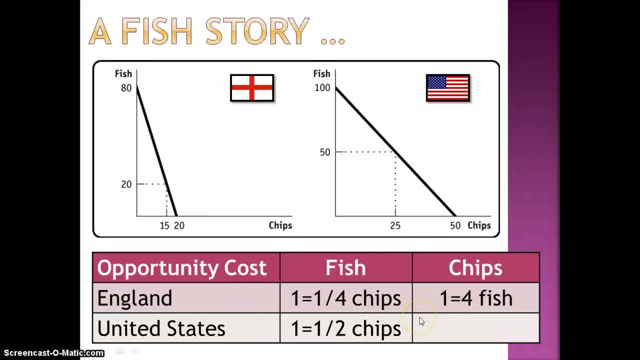 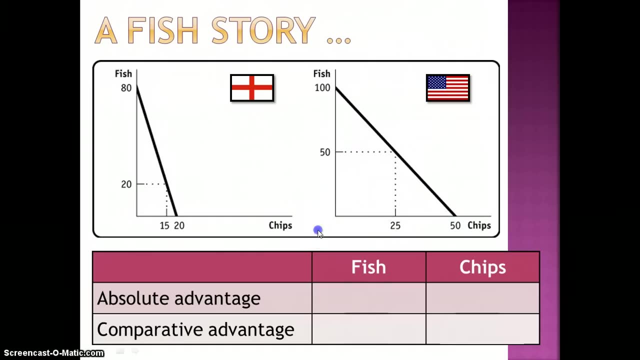 Cost Of one Fish For the US Is one Half Chip That They Make. So We Look At Comparative Advantage Versus Absolute Advantage. We Would Say. 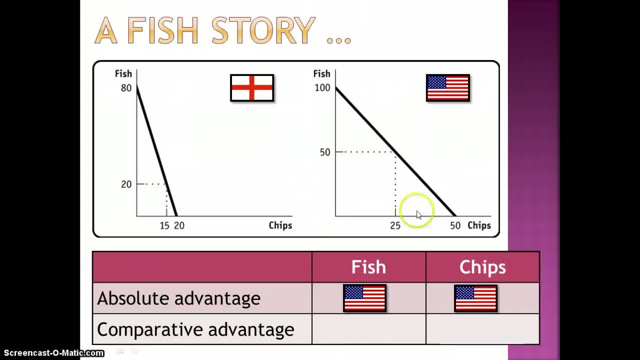 That The Absolute Advantage In Making Fish Belongs To The United States. We Can. England Has A Comparative Advantage In The Production Of Fish Because 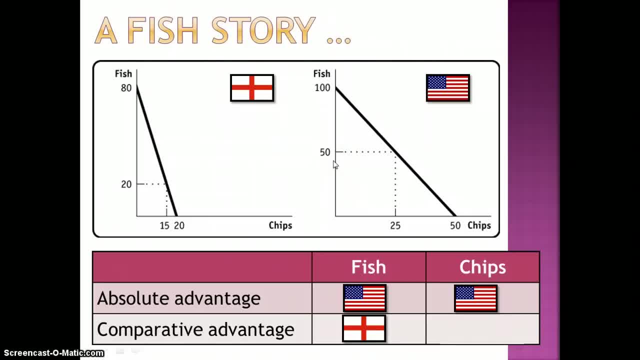 They Only Give Up A Quarter Unit Of Chips For Every Fish They Produce, Whereas The United States Is More Efficient At The Production Of Chips. 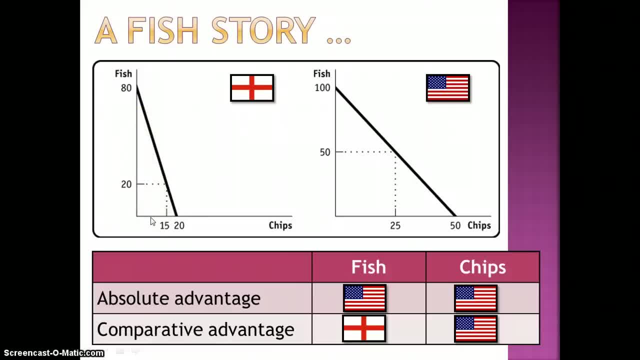 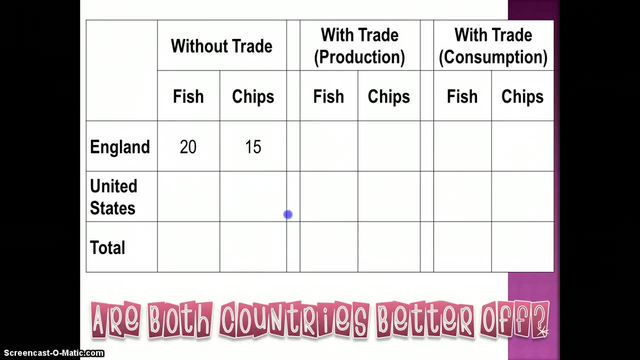 We Give Up Only Two Fish When We Make A Unit Of Chips, Whereas The English Give Up Four Units Of Fish And Twenty Five Chips.